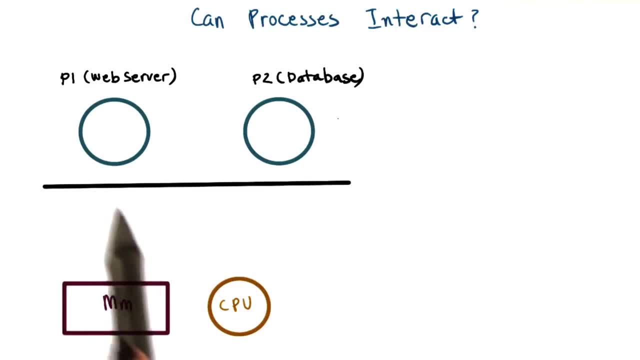 Each of them is a separate address space. They control the amount of CPU each process gets, which memories allocated and accessible to each process. So these communication mechanisms that we will talk about somehow have to be built around those protection mechanisms. These kinds of mechanisms are called inter-process communication mechanisms. 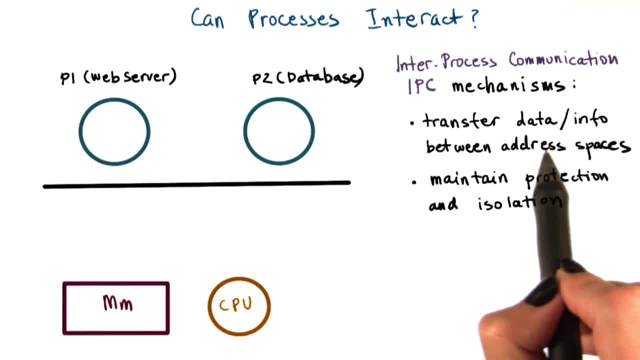 or we refer to them as IPC. The IPC mechanisms help transfer data and information from one address space to another, while continuing to maintain the protection and isolation that operating systems are trying to enforce. Also, different types of interactions between processes may exhibit different properties. 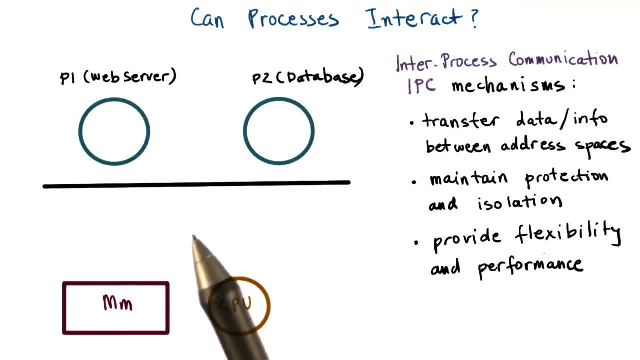 Periodic data exchanges, continuous stream of data flowing between the processes or coordinated update to some shared single piece of information. Because of all these differences, IPC mechanisms need to provide flexibility as well as, clearly, performance. One mechanism that operating systems support is message passing IPC. 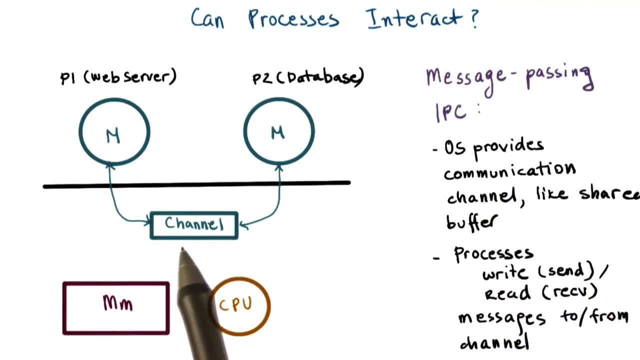 The operating system establishes a communication channel, like a shared buffer for instance, And the processes interact with it by writing or sending a message into that buffer Or reading or receiving a message from that shared communication. So it's message passing, because every process has to put the information that it. 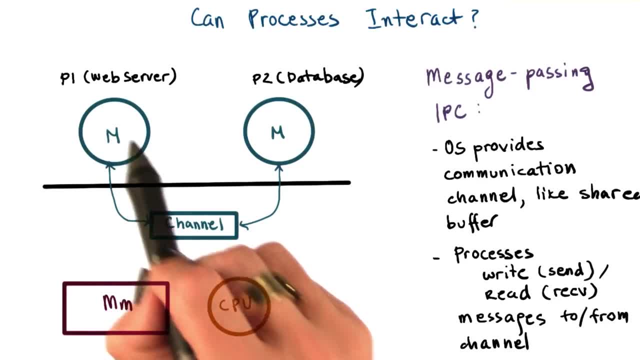 wants to send to the other process explicitly in a message and then to send it to this dedicated communication channel. The benefits of this approach is that it's really the operating system who will manage this channel, And it's the operating system that provides the exact same APIs. 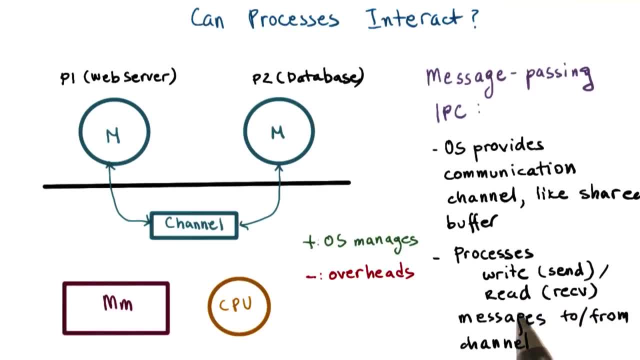 the exact same system calls for writing or sending data and the reading or receiving data from this communication channel. The downside is the overheads, Every single piece of information that we want to pass between these two processes, we have to copy from the user space of the first process. 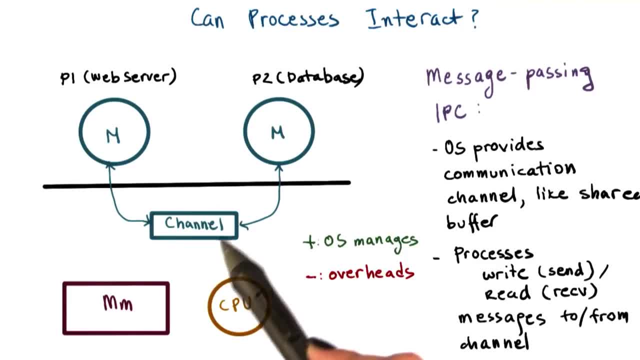 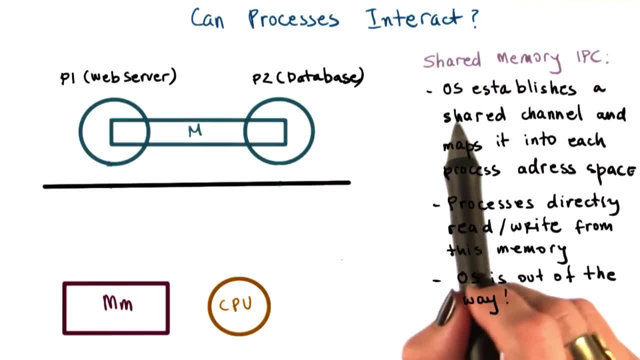 into this channel that's sitting in the OS, in the kernel memory, and then back into the address space of the second process. The other type of IPC mechanism is what we call shared memory IPC. The way this works is that we have a shared memory IPC.